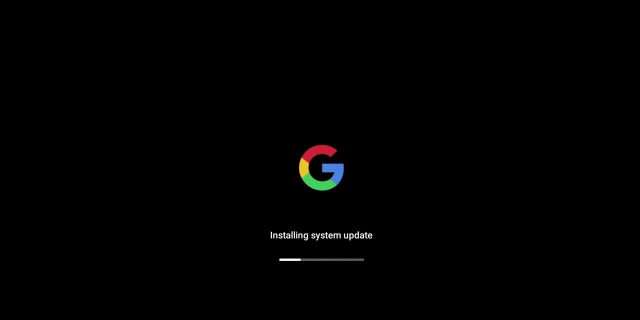 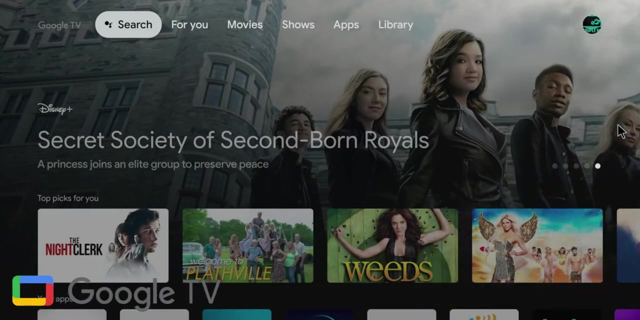 a Chromecast with Google TV. It was the de facto smart TV interface for the new Google Power TVs and set-top boxes And for now, that is the new default smart TV interface for any Google TV, Power TV or set-top boxes that are being released. So if you went to the store and tried to buy 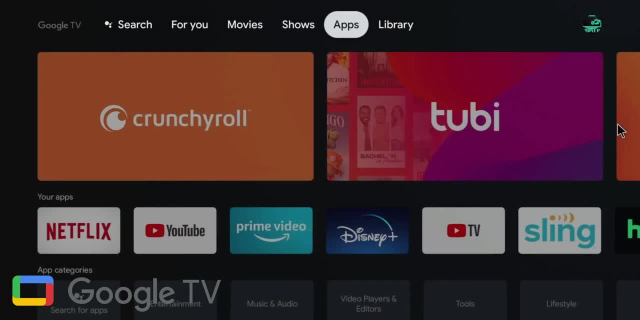 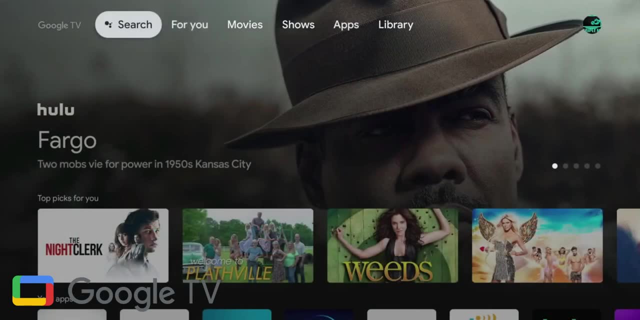 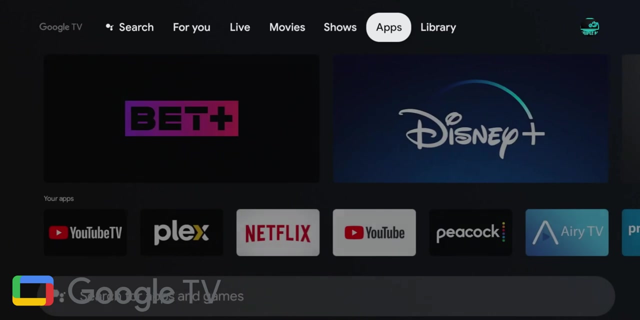 Google TV or Android TV more than likely. if a manufacturer used to come with Android TV, there's a good chance. it's now rolling out Google TV. So what are the main similarities between Google TV and Android TV? So both Google TV and Android TV offer the same selection for smart TV. 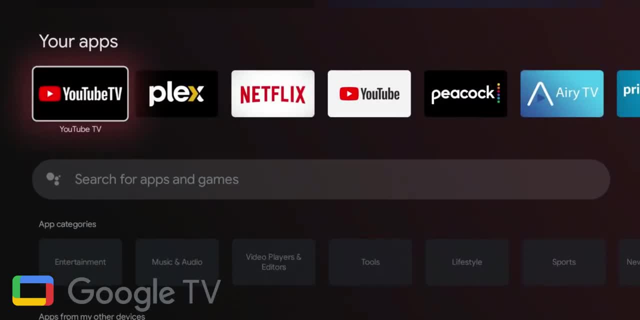 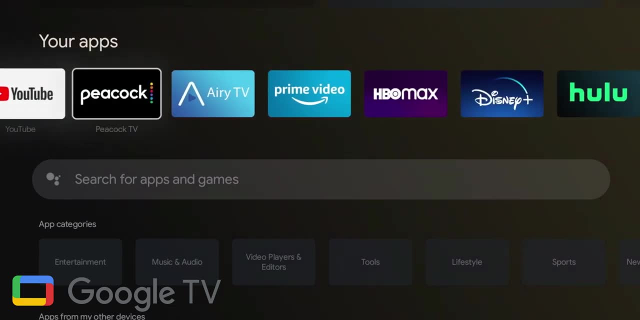 applications games, while also featuring support for voice command with the Google Assistant, smart home controls, casting, Chromecast and media streaming. Both TV systems also offer video games. So what are the main differences between Android TV and Google TV? So, under the hood, they. 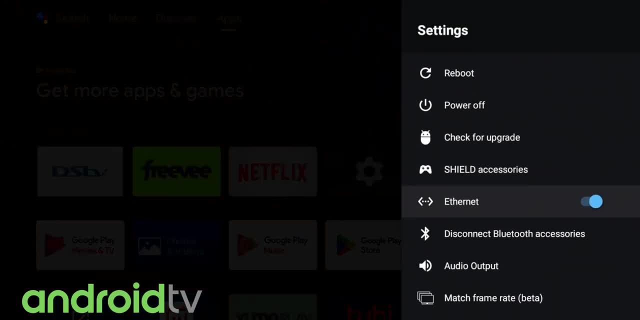 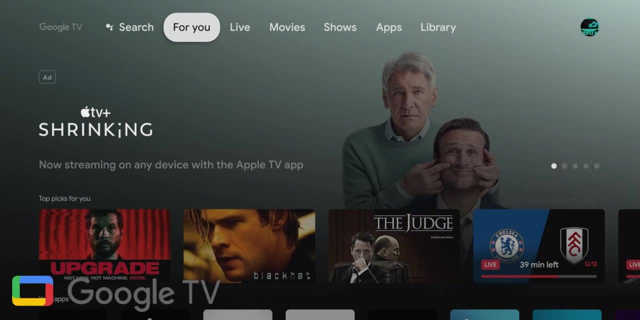 essentially are running the same thing. You can still access the Google Play Store via your app store. You can download pretty much the same applications. You'll get the same quality, But what the main difference is is going to be the user interface. 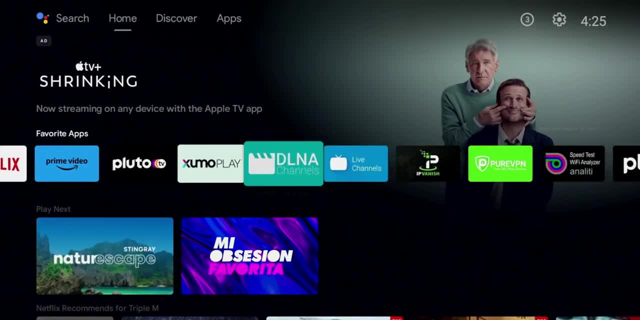 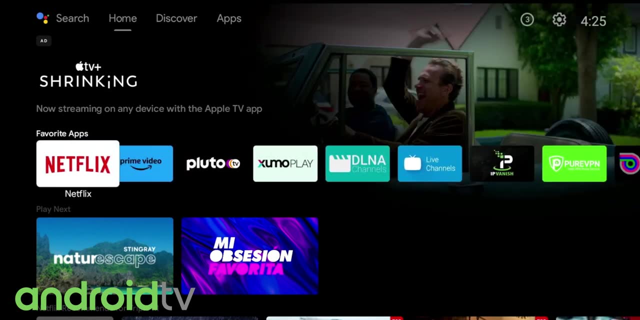 what it looks like on the outside. While Android TV recommendations are based on apps and if you own Nvidia Shield, you're going to see a row of applications. They have made some updates recently, but you'll see, for the most part, applications be recommended or the recommendations. 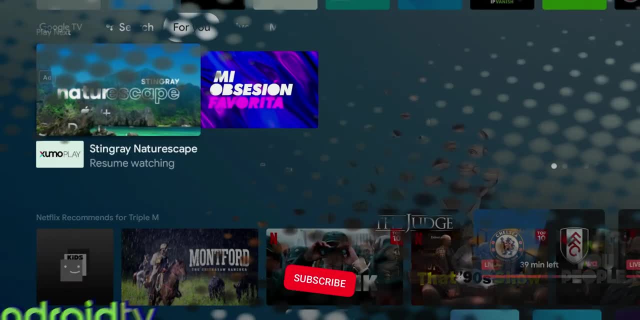 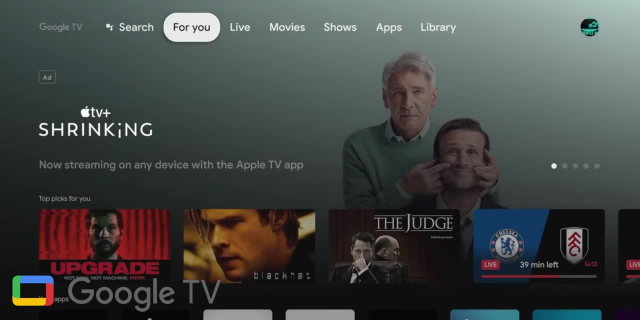 will be based off applications. So what Google does is uses the AI, learns what you like to watch, what you like to look at. The data is then used to make tailored suggestions. on the home screens, dedication for you tab show relevant promotions. 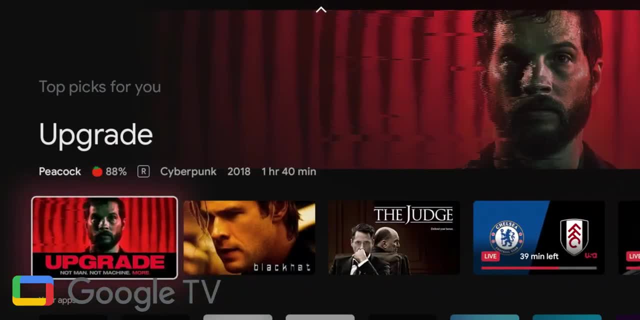 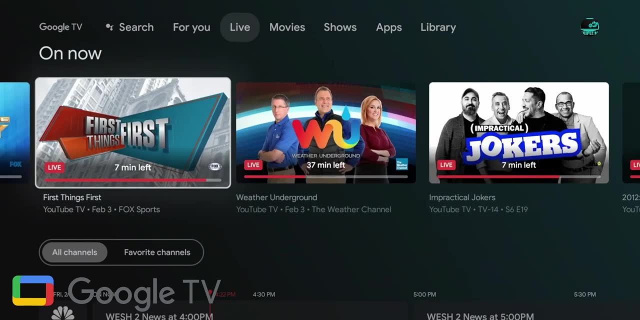 and highlight popular content in your region. Google TV also has a live tab which displays active broadcasts from likes of Sling TV, YouTube TV, So if something piques your interest, simply tap on the thumbnail. go straight to the broadcast. There's no need to open multiple apps. 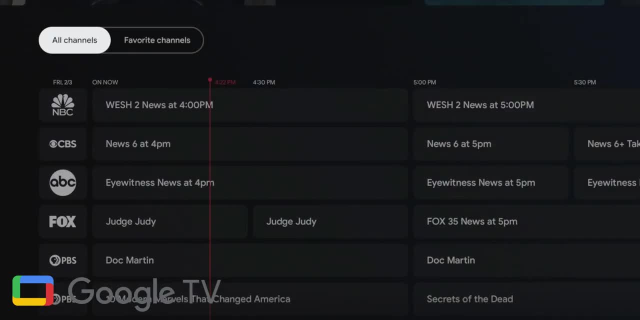 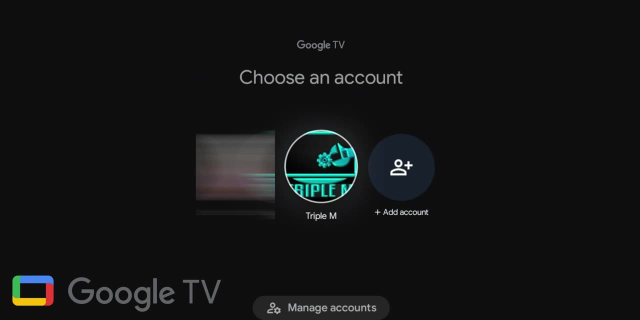 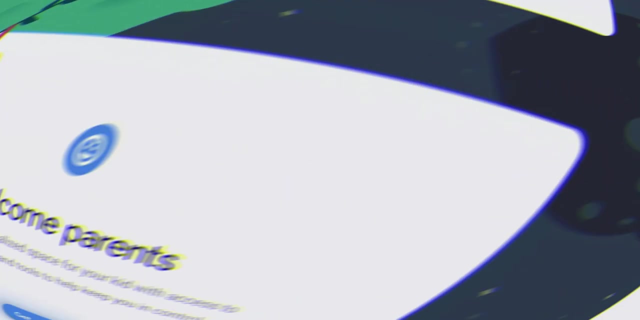 when you find something you want to watch. Another thing that's different between the two is Google TV supports multiple kids profiles on their single adult Google account, with personal recommendations for each profile. Now, while content restrictions on Android TV are handled via its system-wide parental settings, Google TV lets you create child profiles. 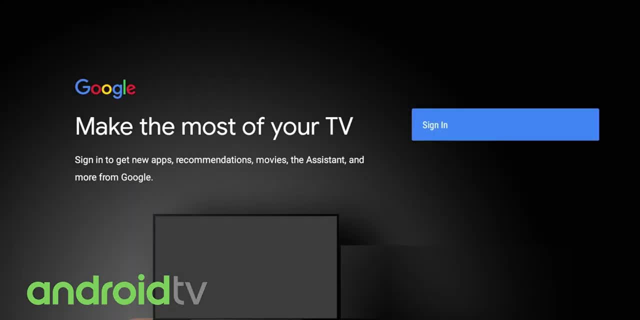 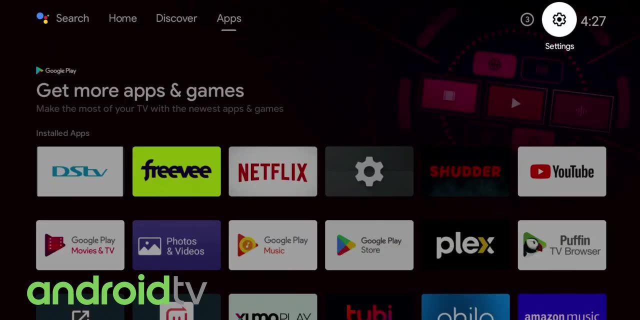 with own set of boundaries for content which can be managed via the Google family link service. So Google goes more in depth, give you more control and essentially lets you control what each account is able to do. So, as I said in the intro, pretty much all. 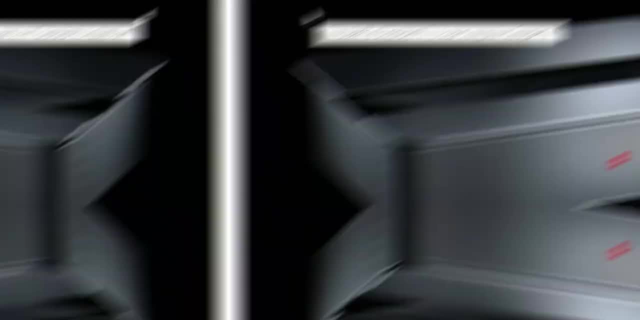 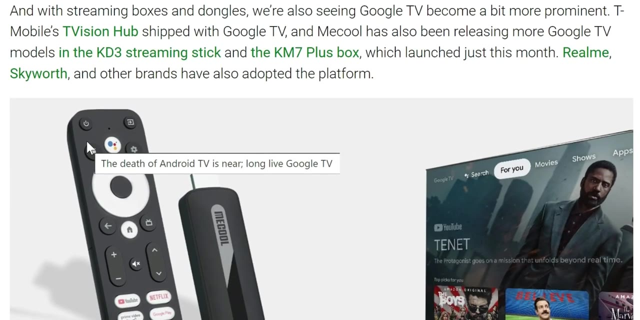 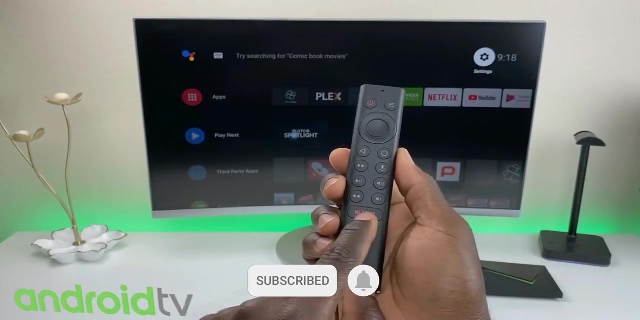 new Google power devices hitting the market, such as the Sony, Bravia and TLC TVs, will be preloaded with Google TV from the outset, but it doesn't look like older Android TVs will be getting an update to a new platform. So for anyone asking about the Nvidia shield, what will happen if? 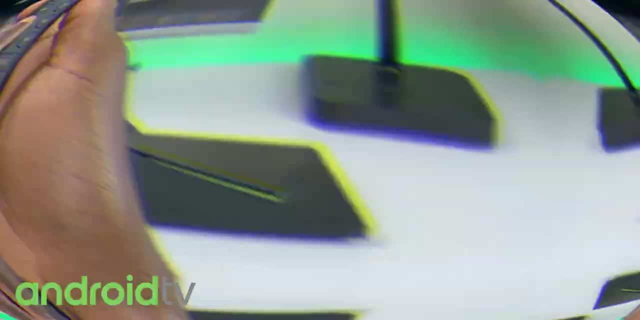 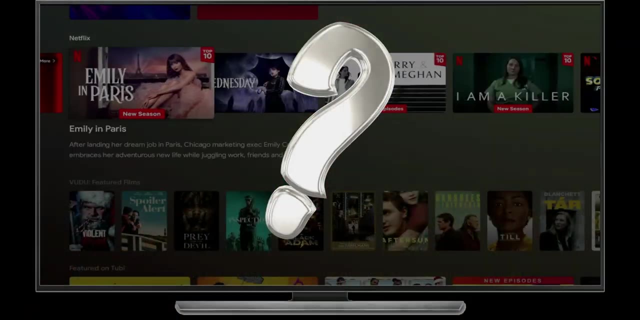 Android TV stopped rolling out. I don't think for one that they'll stop pushing updates and they will not upgrade it to the Google TV, but I just think that new products coming out, whether it's a new Nvidia Shield, which we are due for, 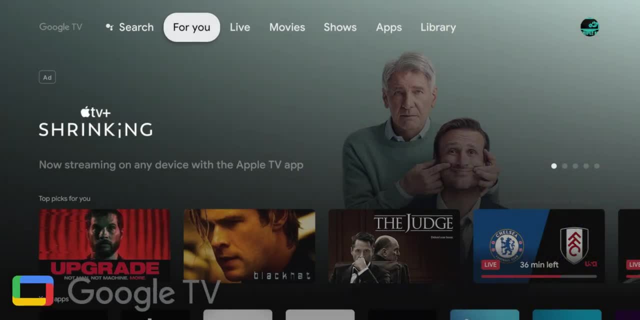 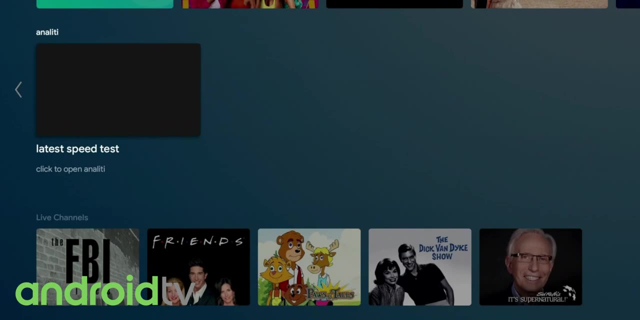 might see that Google TV UI pop up in it. So in the end, not a big deal to me. In my opinion, Android TV have more options as far as customizing what you want to see on the homepage. Google TV, like I said, it uses more of that AI knowledge. 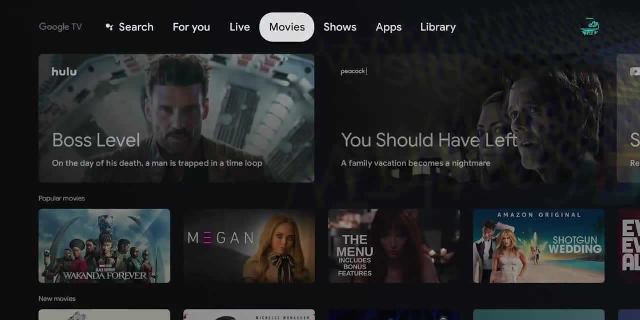 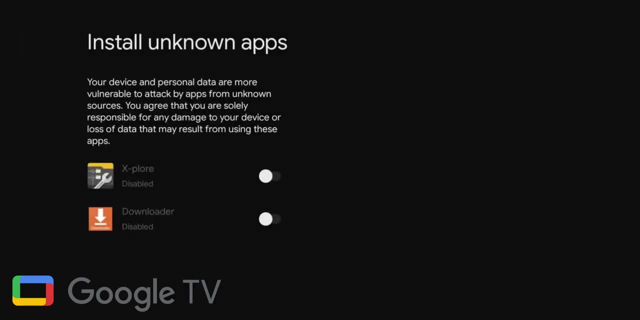 to recommend what they think you wanna watch, And the interface on Google TV is a little bit cleaner, in my opinion, but under the hood you still get the same accessibility options, ability to download third-party applications, as well as the ability to access the applications. 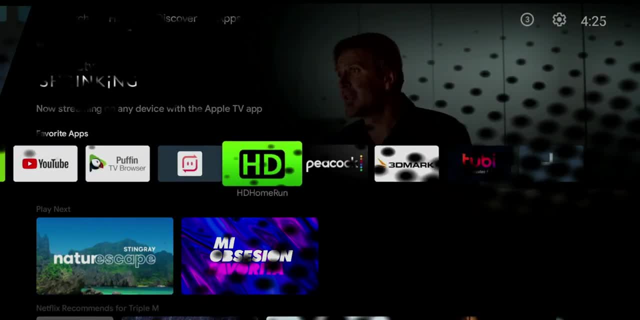 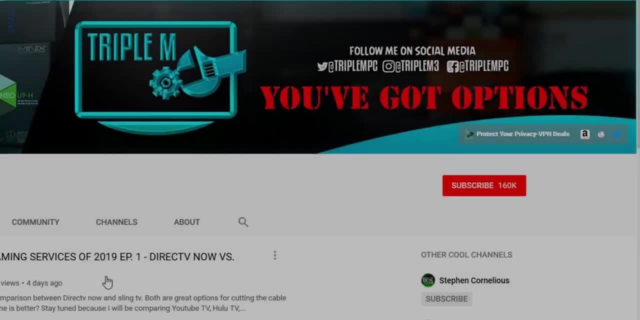 on the Google Play Store. So in the comment section let me know what you guys think. Let me know if this kind of cleared it up a little bit for you. In my opinion they're definitely more similar than they are different If you're new to the channel. 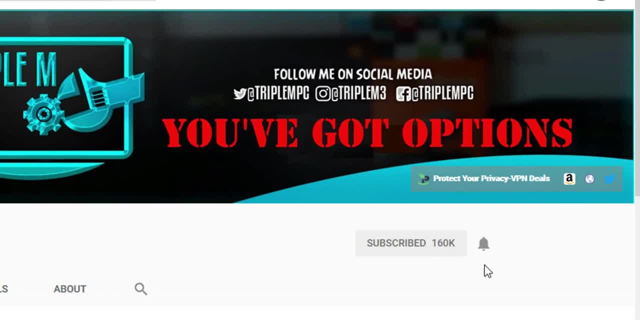 subscribe. smash the notification bell. Thank you for watching and I'll catch you on the next one. 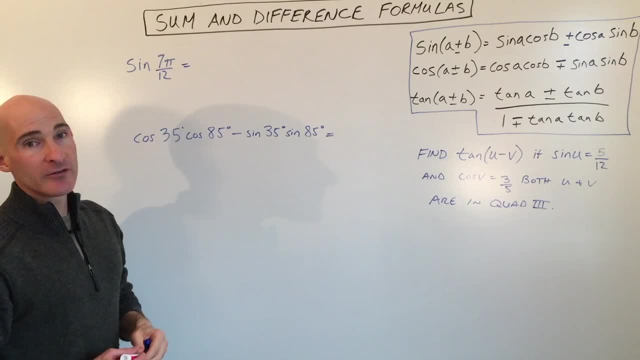 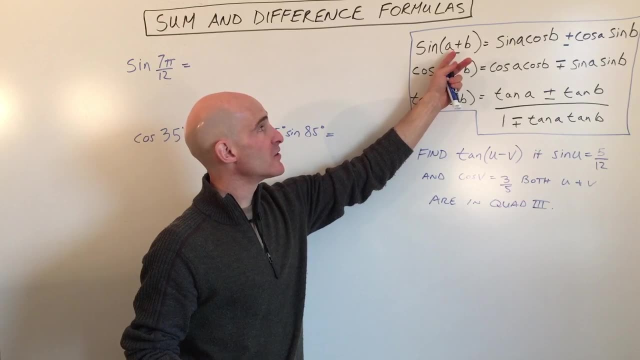 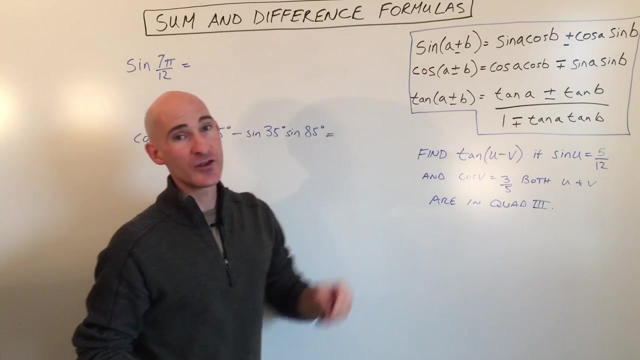 Let's say you want to find out sine of 7 pi over 12.. Now this isn't one that we memorized on the unit circle. so what we can do is we can take two angles that either add or subtract, to give us 7 pi over 12 using those two angles that we know on the unit circle. So sometimes students